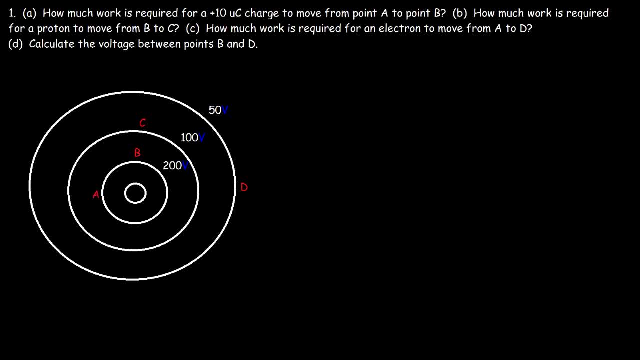 In this video we're going to focus on equi-potential lines and surfaces, But let's start with this problem: How much work is required for a 10 microcoulomb charge to move from point A to point B? So how much work is required to move it from here to here? 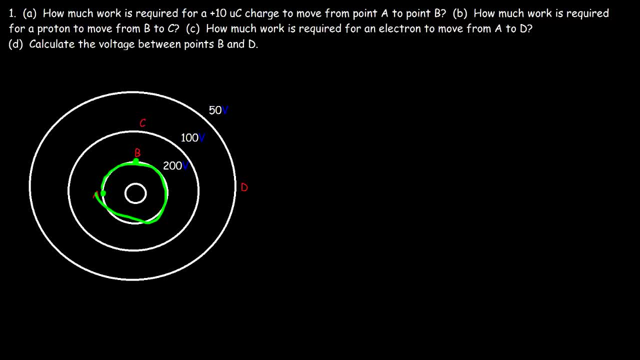 Now notice that we have an equi-potential line. In the case of a sphere it would be an equi-potential surface. Notice the electric potential is the same anywhere along that equi-potential line. So at A and at B the electric potential is 200 volts. 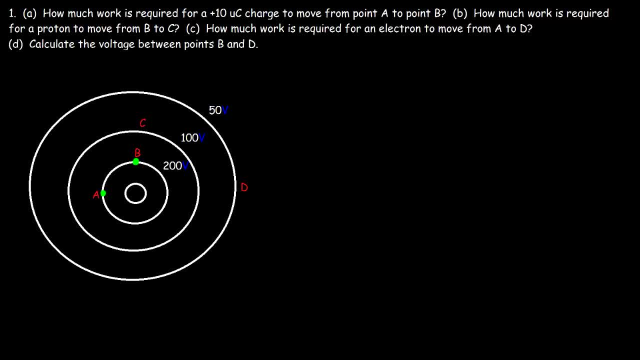 So there is no potential difference. As a result, there's no work required to move a charge along an equi-potential line or an equi-potential surface. So to move it from point A to B, no work is required because the electric potential is still the same. 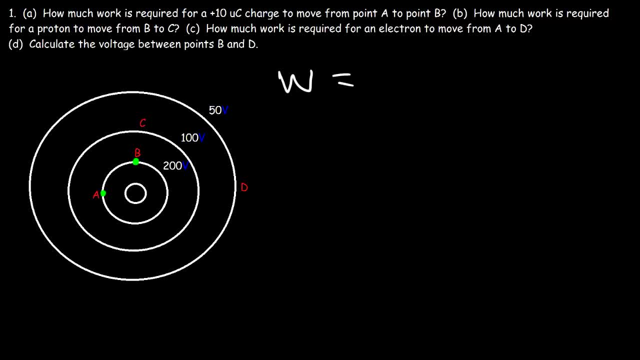 To calculate the work required to move a charge from one potential to another. here's the formula that you need: It's negative Q delta V. So in this case we have a positive 10 microcoulomb charge And micro is 10 to negative 6.. 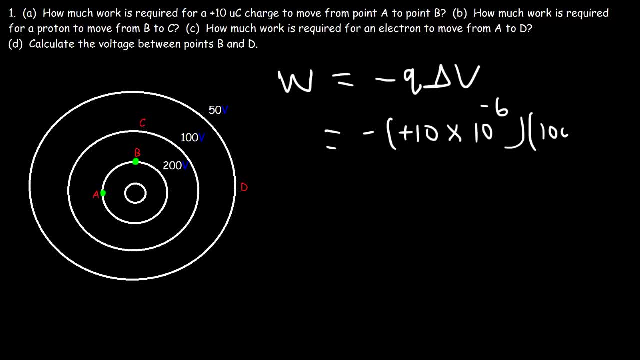 Now the potential at point B is 100. And the electric potential I mean it's 200 rather not 100. It's this number. The electric potential at point A is also 200 volts. So the change in potential or the voltage is zero between those two points. 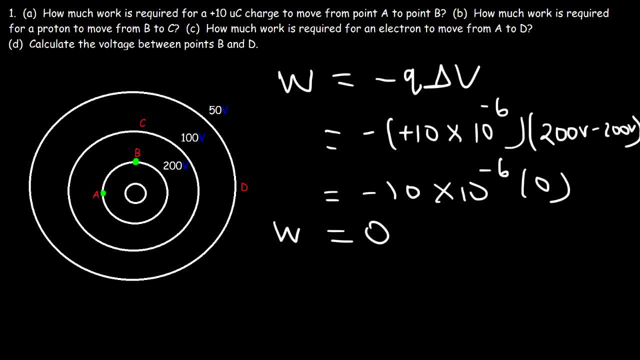 So whenever you multiply anything by zero, the whole thing is zero, So no work is required to move a charge along an equi-potential line or surface. Now, chances are there's a positive charge at the center, Since we have positive electric potentials around that charge. 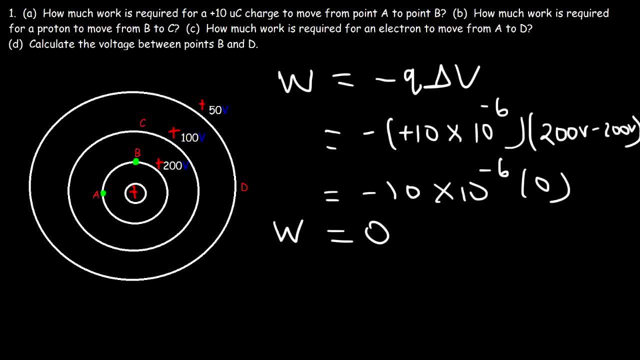 Now let's move on to part B. How much work is required for a proton to move from B to C? So this time the electric potential is changing, So work is going to be required to move the charge from B to C, And so we can calculate it. 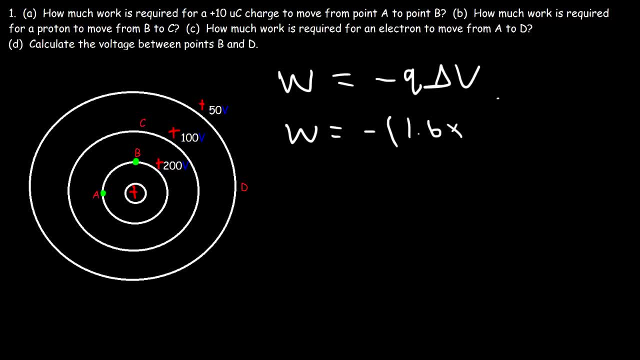 The electric charge of a proton is positive 1.6 times 10 to the negative 19 coulombs And the change in potential going from B to C. the final electric potential is 100 volts. The initial is 200.. 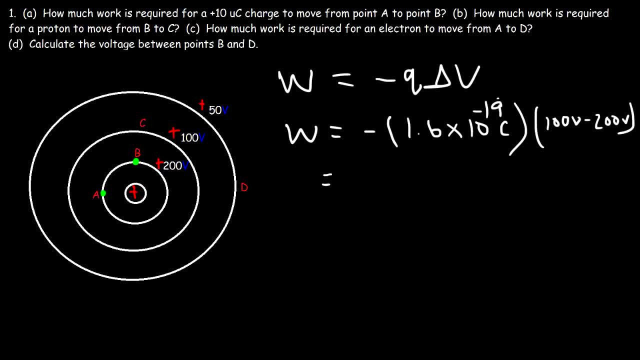 And so the change in electric potential, or basically the voltage, is negative 100 as we go from B to C. So notice that the work required to move a positive charge is negative 100 volts. So notice that the work required to move a positive charge. 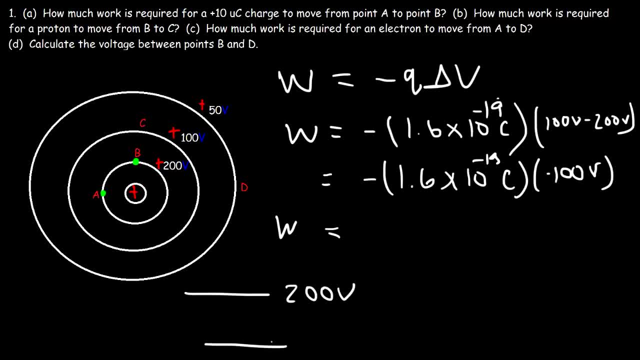 from a high potential to a low potential is positive. So as this positive charge goes from a high voltage to a actually high electric potential, to a low electric potential, the work done on the charge is positive, Which means that the charge is accelerating. 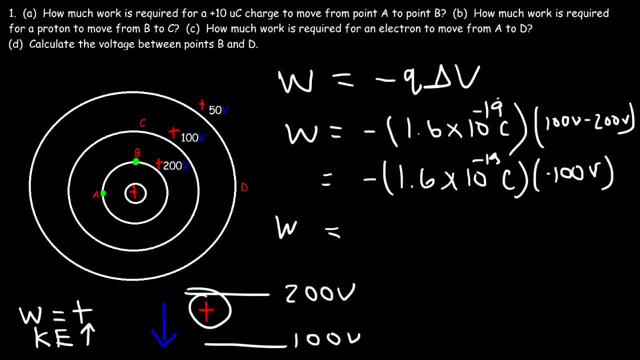 It's going to speed up. The kinetic energy of that charge is increasing. Now let's go ahead and get the answer. So it's 1.6 times 10 to the negative, 19 times 100.. And so this is going to be positive 1.6 times 10 to the negative: 17 joules. 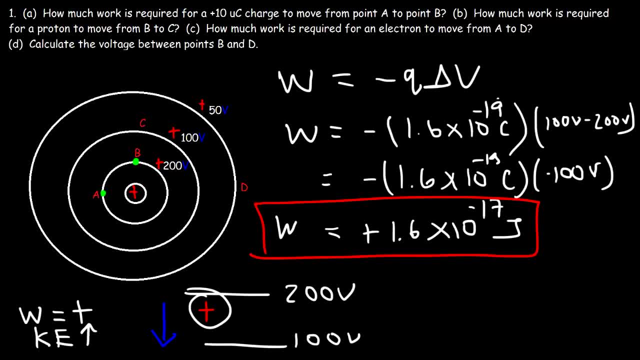 Now, if you want to see how the units work in this example, Q is in coulombs, Volt. one volt is a joule per coulomb, So the unit coulombs cancel, and so you get the unit joules. 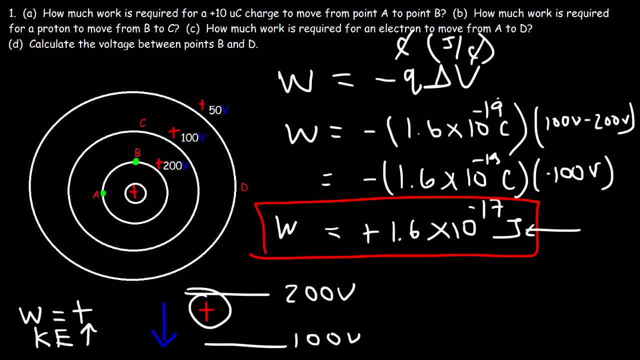 Now what about part C? How much work is required for an electron to move from A to D? So the electron is moving from a high potential to a low potential, So it's displacement is in this direction. Will the work be positive or negative? 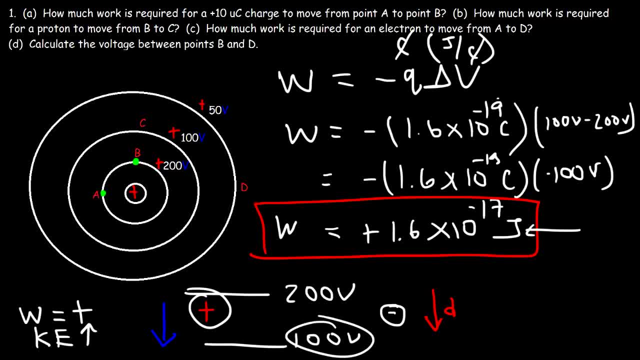 Now, anytime an electron is moving towards a lower potential or towards a negative charge, it's going to feel a force that's going to accelerate in the other direction, And whenever force and displacement are opposite to each other, the work done is negative. 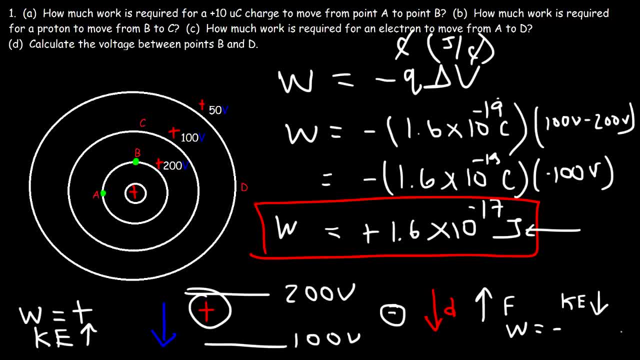 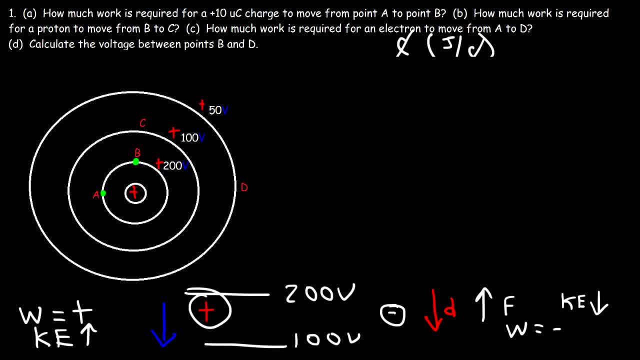 which means that the kinetic energy of the electron is decreasing, It's slowing down. So we should get a negative answer. But let's see how much we should get. So let's use the same formula. Work is equal to negative. Q, delta V. 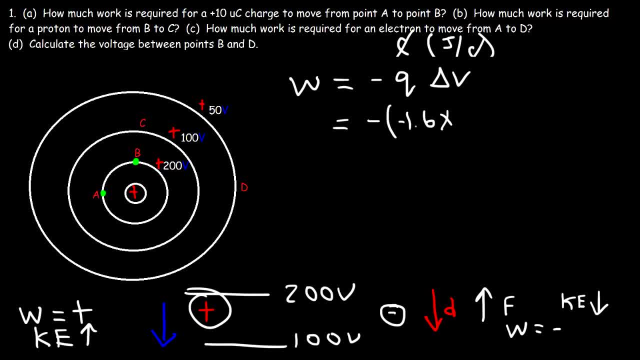 So the charge of an electron is negative 1.6 times 10 to the negative 19 coulombs And we're going from A to D. So the electric potential at D is 50.. That's the final potential minus the initial potential at A, which is 200. 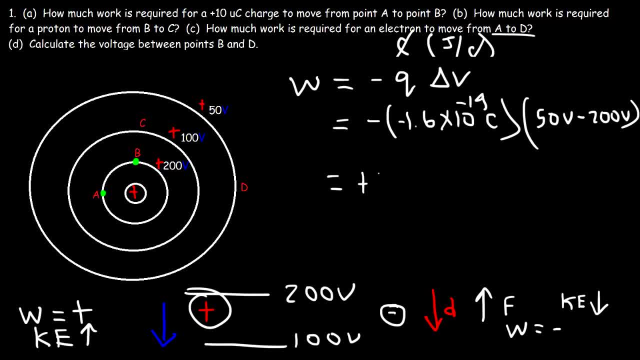 So these two negatives will create a positive sign. So that's positive 1.6. And then 50 minus 200, that's negative 150 volts or negative 150 joules per coulomb, And so we can cancel So these units, and so we can see why it's going to be a negative value. 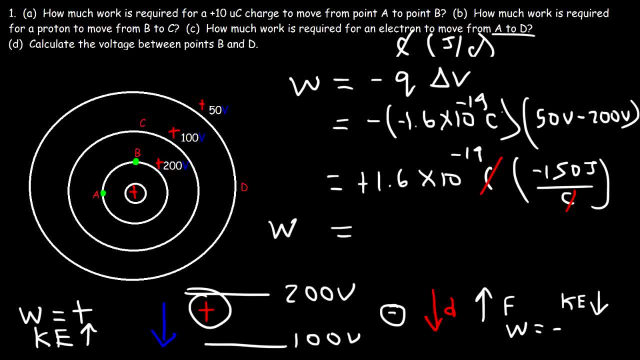 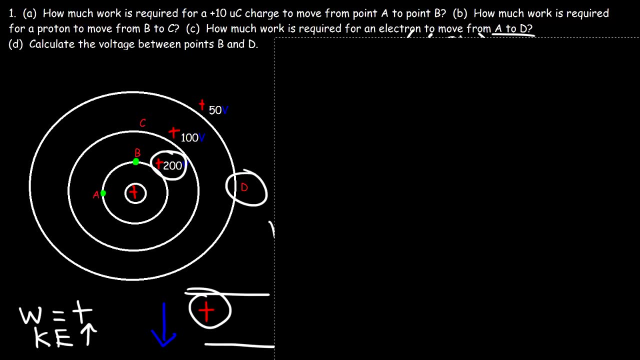 And so the work required to move an electron from A to D is negative 2.4 times 10 to the negative 17 joules. And so that's the answer for part C. Now calculate the voltage between points B and D. The voltage is simply the potential difference. 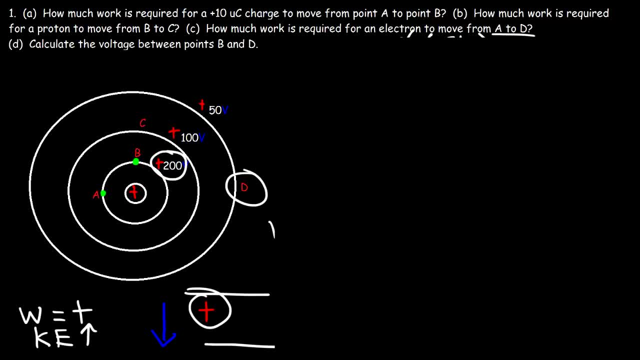 It's the difference in the electric potential of two points. So if we're traveling from B to D, the electric potential is decreasing. The final value is 50.. The initial value is 200.. So the change is negative 150 as we go from B to D. 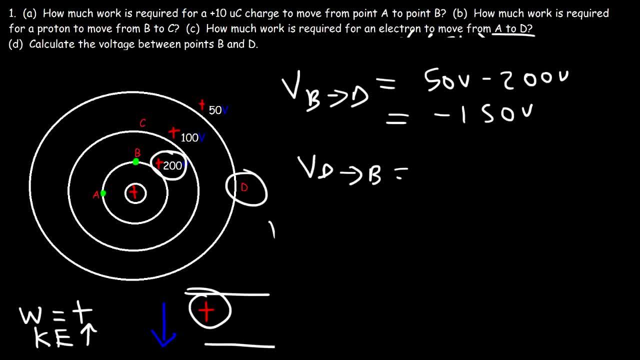 Now, if we're going from D to B, The final value is 200, and the initial value is 50. So, as you can see, the voltage between those two points can be positive 150, or it can be negative 150. 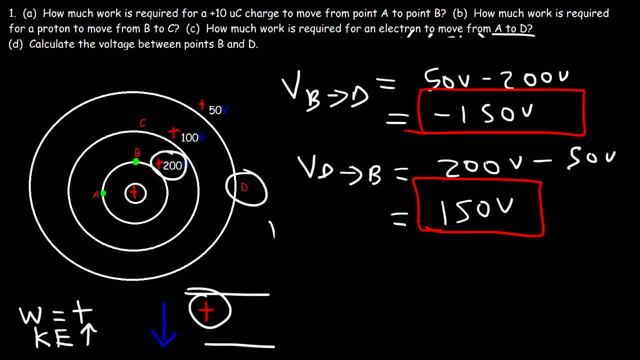 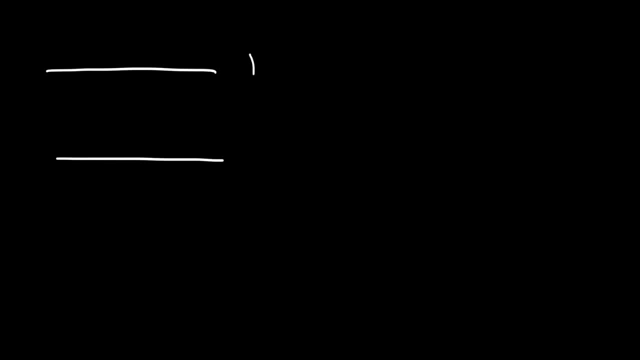 And it all depends on the direction in which you're moving. But that's the difference between points B and D. It differs by 150 volts, So you could say it's negative 150 or positive 150.. Now consider this problem. Let's say if we have two equipotential lines and the electric potential for these two lines. 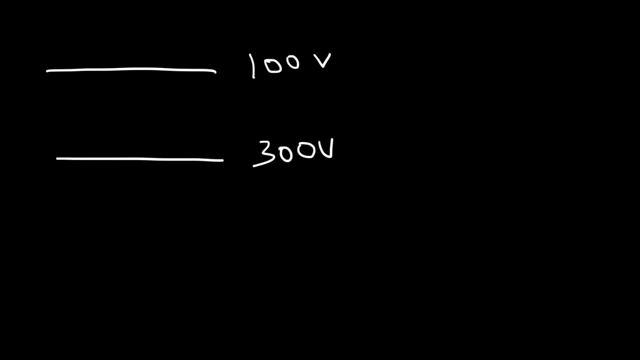 are 100 volts and 300 volts. What is the direction of the electric field? The electric field is always perpendicular to an equipotential line and it travels from high potential to low potential, the same way as a ball travels from a high position. 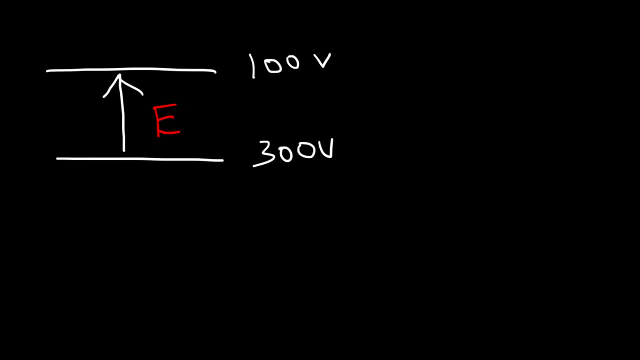 and falls to a lower position, And so the electric field is directed In a positive y direction. Now let's say if the distance between these two lines, let's say if it's 4 meters, What is the magnitude of the electric field? 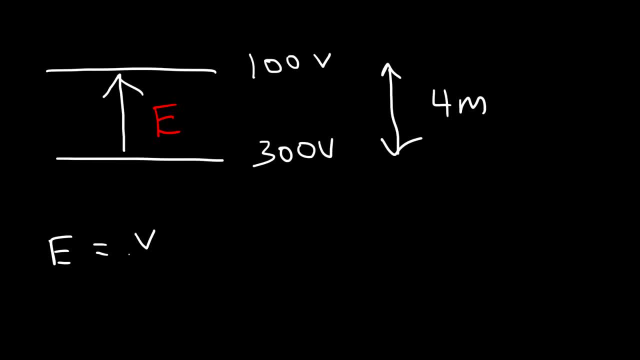 The electric field is simply the voltage, which is the change in the electric potential divided by the distance. So the voltage or the difference between these two values 300.. 300 minus 100 is 200 volts And D is 4.. 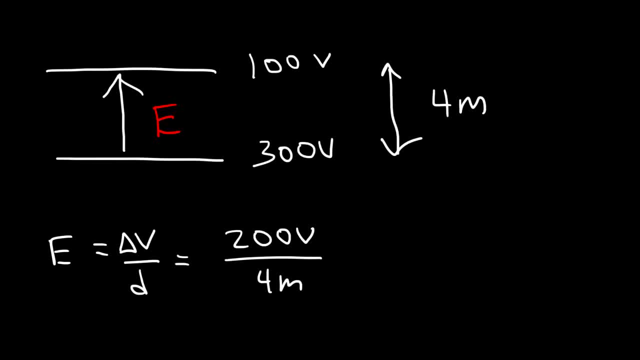 Now you could adjust the sign. Sometimes it could be positive, sometimes it could be negative. Now the electric field is going in a positive y direction, So we can assign a positive value to it. Now I believe this equation is actually supposed to have a negative sign. 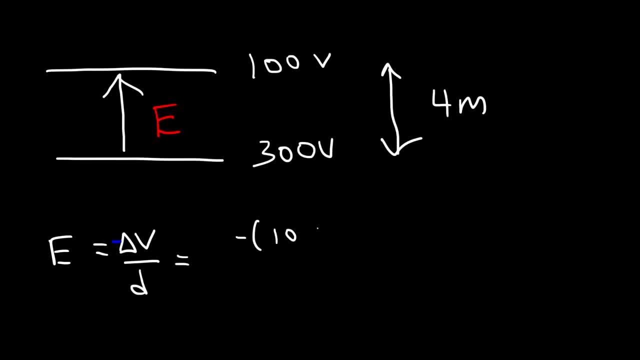 And so the final value is 100.. The initial value is 300.. So in the end you should still get a positive value. So this is going to be negative times negative 200, divided by 4 meters, And so the electric field is going to be 50 volts per meter. 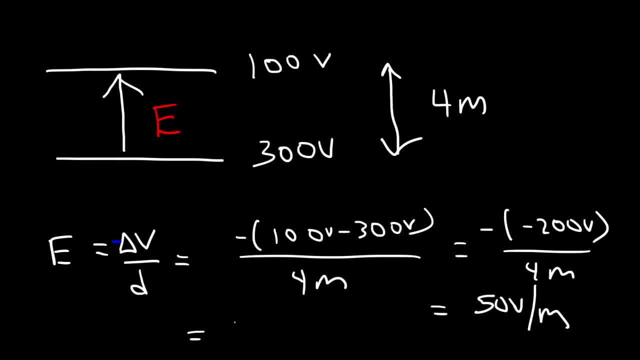 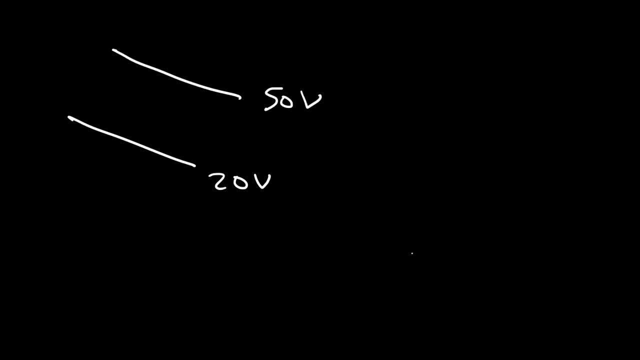 So you can call this a potential gradient. Now you can also use the units Newtons per Coulomb. The electric field can be described in both ways. Thank you. Now go ahead and try these two. Draw the direction of the electric field. 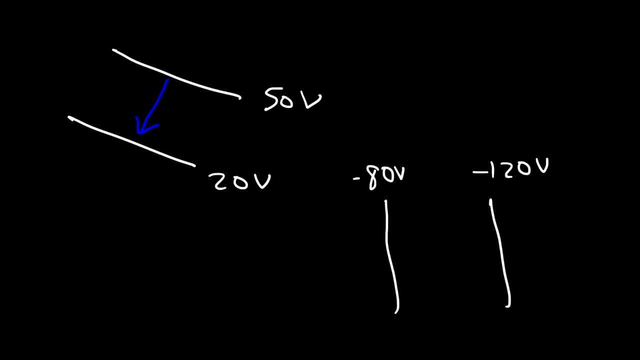 So the electric field always points from a high potential to a low potential, So it's going in this direction And make sure that it's perpendicular to the equipotential line. Now which number is higher? Negative 80 or negative 120?? 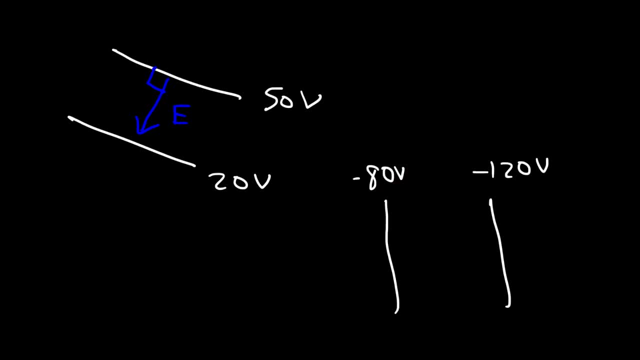 Negative 120.. Negative 120. on a number line, Negative 80- is higher than negative 120.. On a number line, let's say this is 0,, this would be negative 80, and over here, this would be negative 120. 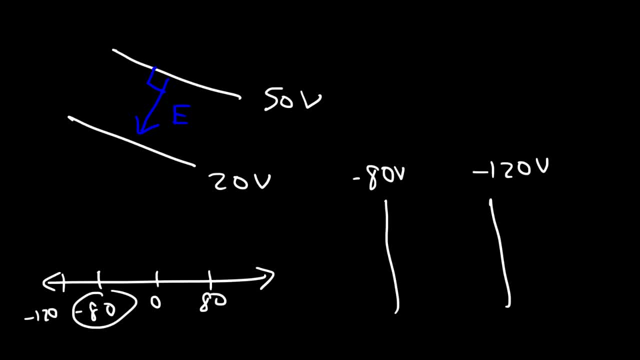 And this would be positive 80.. So negative 80 is to the right of negative 120, so it's higher in value. So therefore, the electric field is going to go from the high potential to the low potential, So it's directed east or to the right.